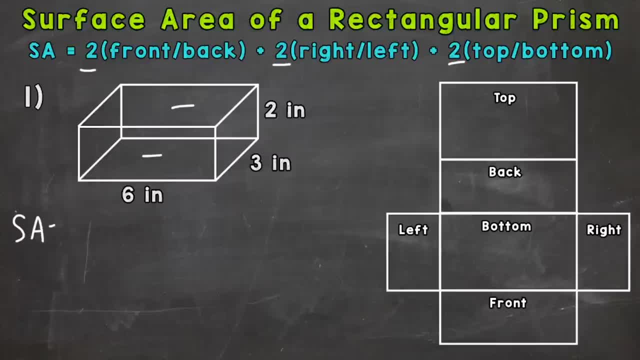 here And we'll start with surface area equals two And we need to find the area of the front or back. So let's find the area of the front where we have a six by two, So we can do: area equals length times width for a rectangle. Plug in Area equals. 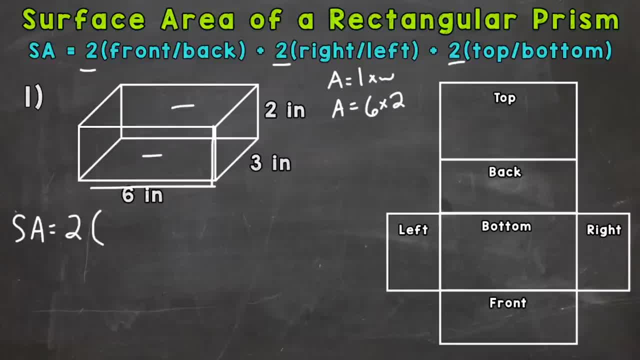 six times a width of two And we get an area of 12 square inches for the front. So we could plug in 12 here Plus now. we need to do the right and left Now. but before I get to that, 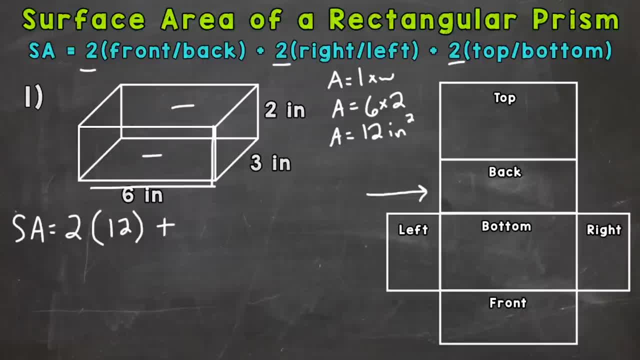 I want to mention to the right here. I have a net of that rectangular prism, So basically I unfolded it so you can see all of the faces, And it's not in 3D form, So it kind of lays everything out. so we 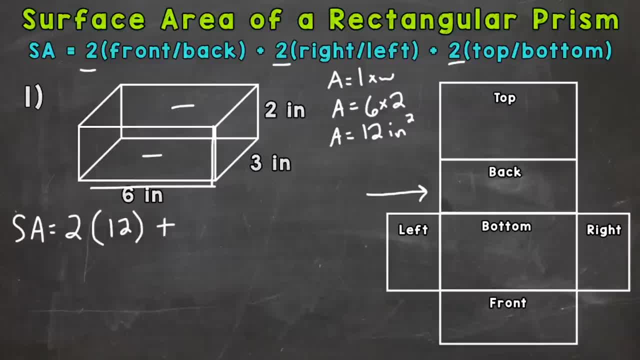 can visualize what we're doing a little better. So, as of right now, we have 12 square inches Here for the area of the front and the back. So let's do right and left, So we'll pick the right side here, the right face, and we have a three by two. 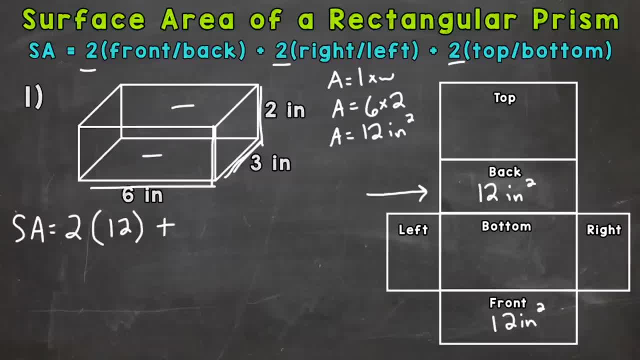 So area equals length times width. So we can plug in three times two And that gives us an area of. let's actually write it out: Length times width, Area equals three times two. So that area is going to be to be six square inches. so again, that's the right and left. so we would do two times six for the. 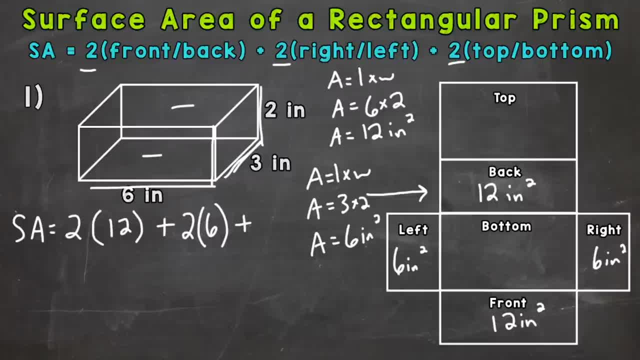 right and left and lastly, we need to do the top and the bottom. so we're going to take a look at the top, where we have a six by three, so area equals length times width. plug in six times three and we get an area of 18 square inches. so our bottom is 18 square inches and our top 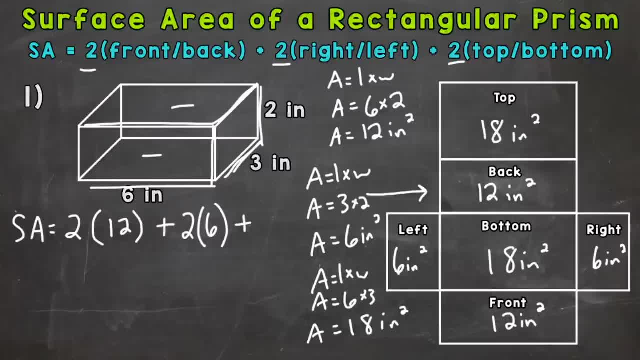 is 18 square inches, so we would plug in two times 18.. Now let's start solving: two times 12 is 24, two times six is 12, plus two times 18 is 36, so the top or, I'm sorry, the front and back combined. 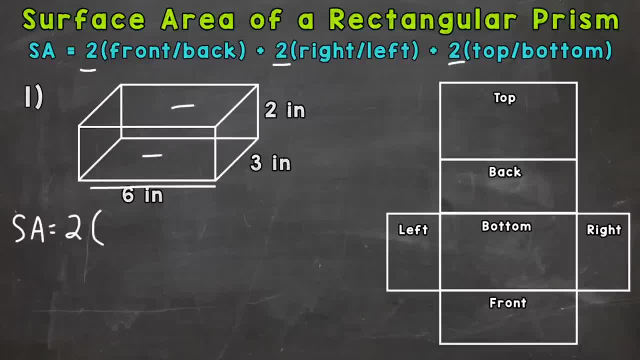 have a six by two so we can do: area equals length times width for a rectangle plug in. area equals six times a width of two and we get an area of 12 square inches plus for the front. so we could plug in 12 here plus now. we need to do the right and left now, but before. 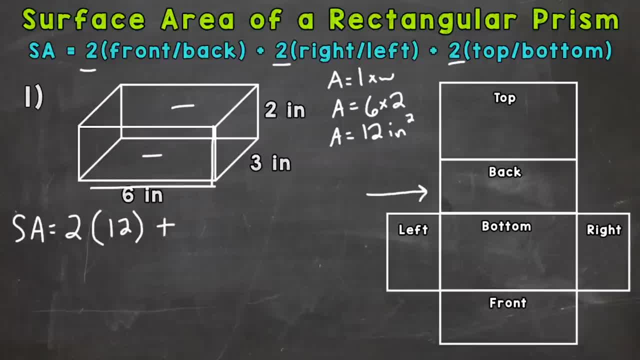 i get to that. i want to mention to the right here i have a net of that rectangular prism, so basically i unfolded it so you can see all of the faces, um, and it's not in 3d form, so it kind of lays everything out so we can visualize what we're doing a little better. so, as of right now, we have 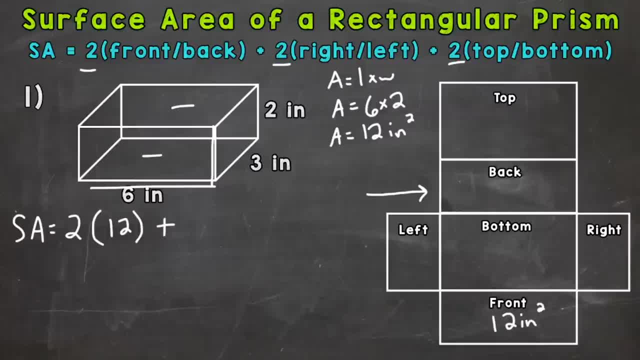 12 square inches here for the area of the front and the back. so let's do right and left, so we'll pick the right side here, the right face, and we have a three by two. so area equals length times width. so we can plug in three times two and that gives us an area. 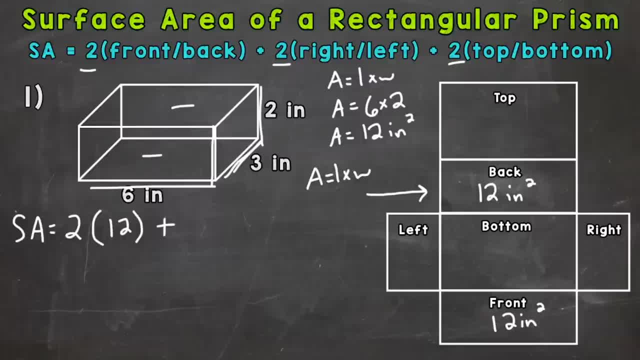 of. let's actually write it out: length times width area equals three times two, so that's the area of the front, and the back area is going to be six square inches. so again, that's the right and left. so we would do two times six for the right and left. and lastly, we need to do the top and the. 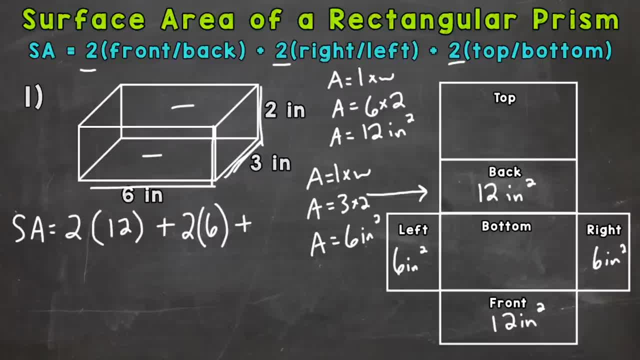 bottom. so we're going to take a look at the top, where we have a six by three. so area equals length times width. plug in six times three and we get an area of 18 square inches. so our bottom is 18 square inches and our top is 18 square inches. so we would plug in 2 times 18..